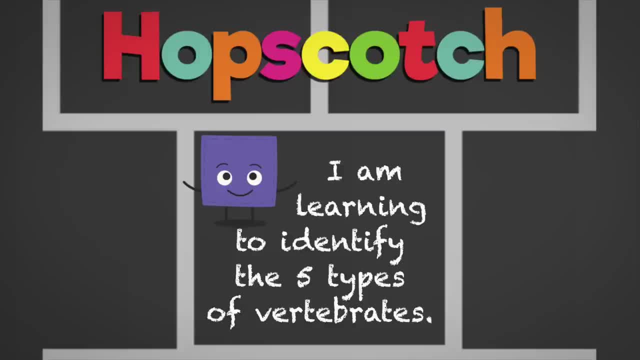 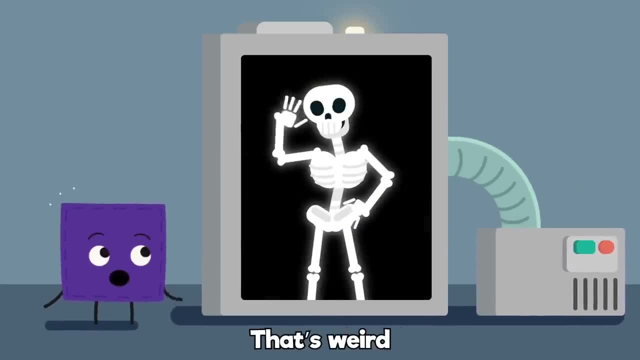 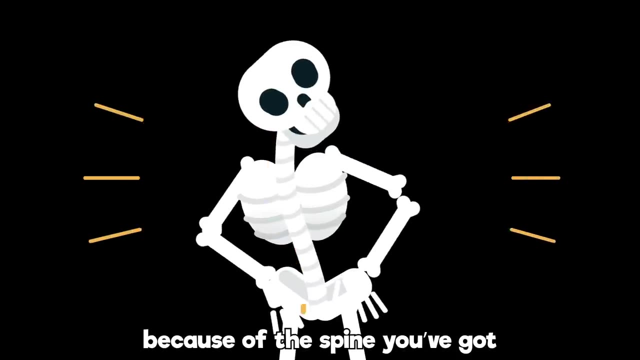 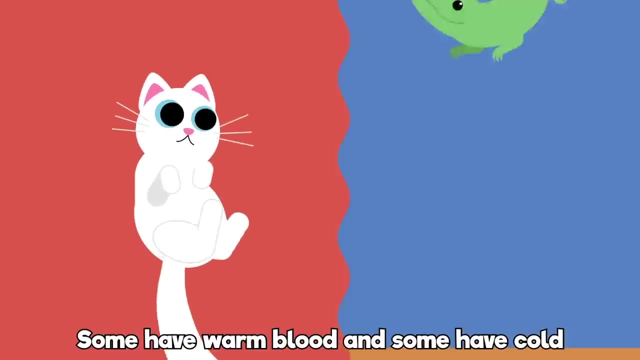 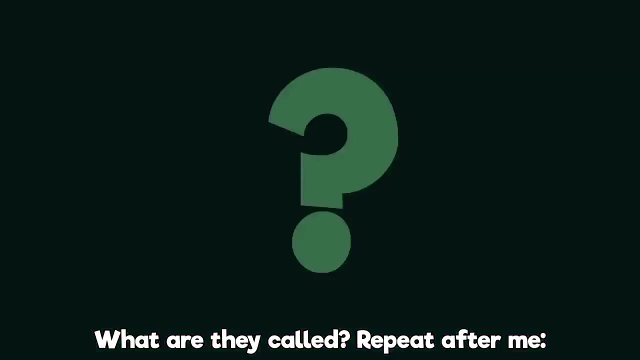 Do you have a backbone? That's weird. 95% of Earth life does not. You're called a vertebrate because of the spine you've got. Verify vertebrate classes. Some have warm blood and some have cold. Some aren't landing in the air or sea. What are they called? Repeat after me. 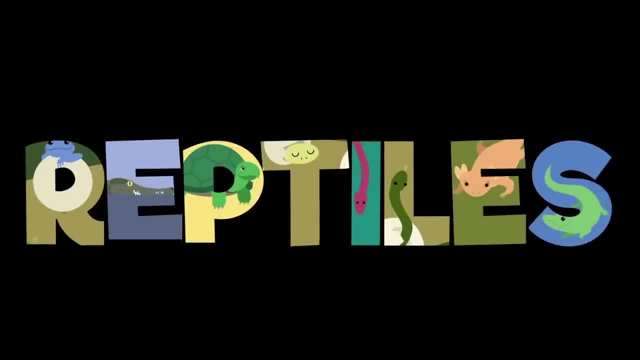 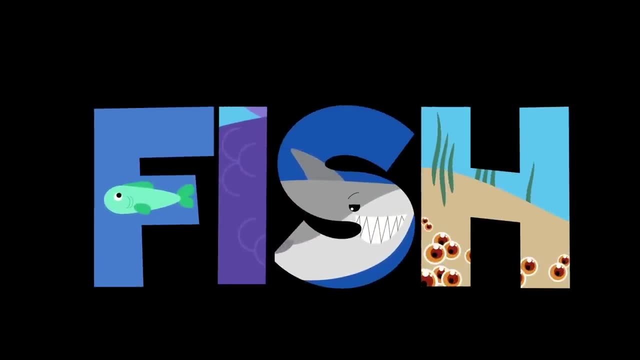 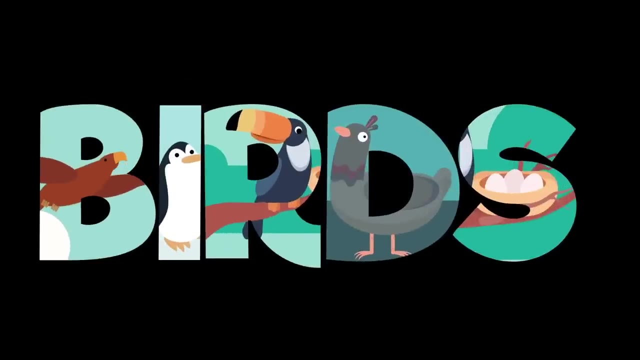 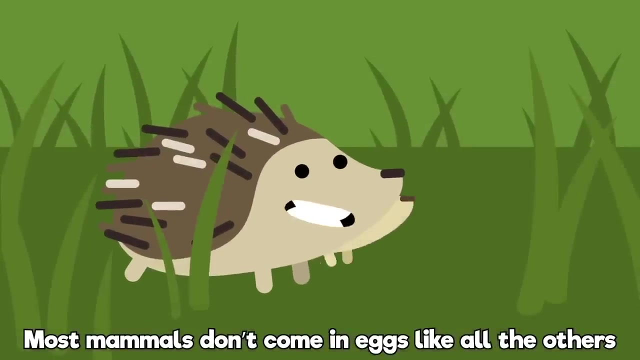 Mammals, reptiles, birds, amphibians and fish. Mammals, reptiles, birds, amphibians and fish. Most mammals don't have a spine. They don't come in eggs like all the others. The babies drink milk from their mothers. 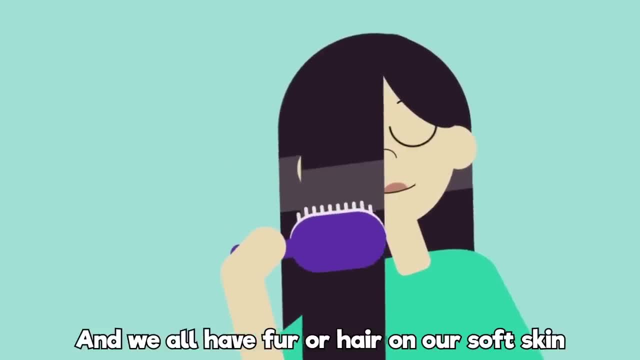 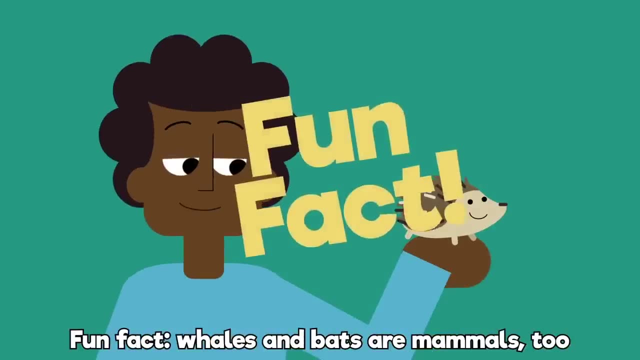 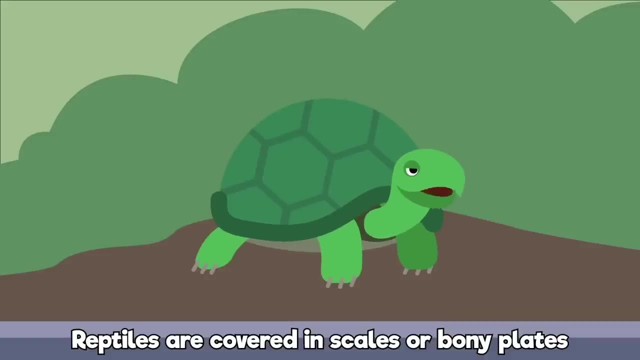 And we all have fur or hair on our soft skin. We have cats, deer, platypus, kangaroos and you. Fun fact, whales and bats are mammals too. Reptiles are colored in scales or bony plates. 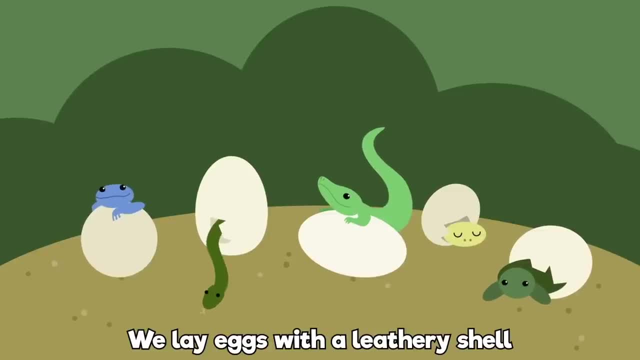 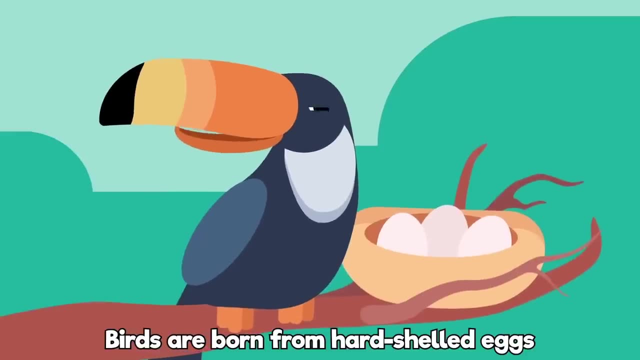 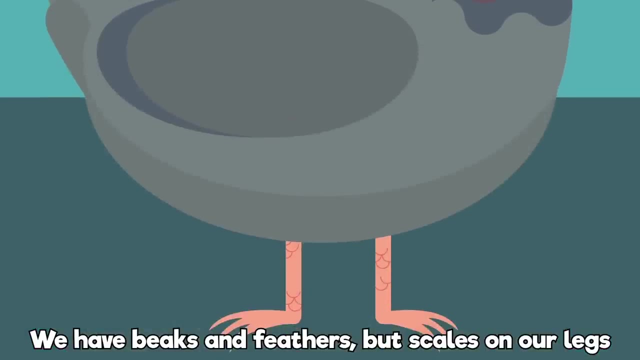 Yeah, we know you can't relate. We lay eggs in the lake. We have a feather, a shell, We have snakes, lizards, crocodiles and turtles as well. Birds are born from hard-shelled eggs. We have beaks and feathers, but scales on our legs. 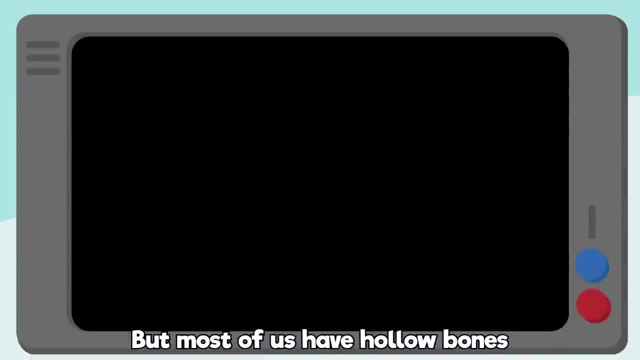 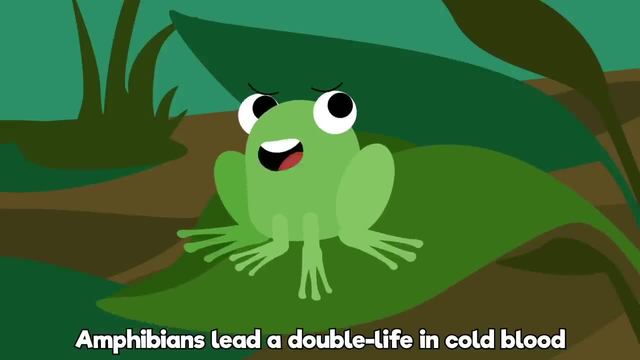 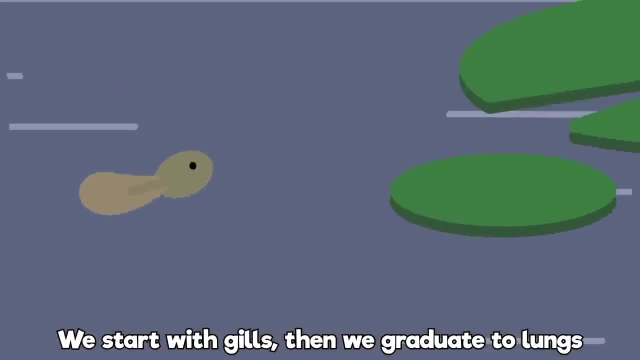 Not all of us take to the sky, But most of us have hollow bones and most of us fly. Amphibians lead a double life in cold blood, But our metamorphosis takes us from the water to the mud. We start with gills, then we graduate to lungs. 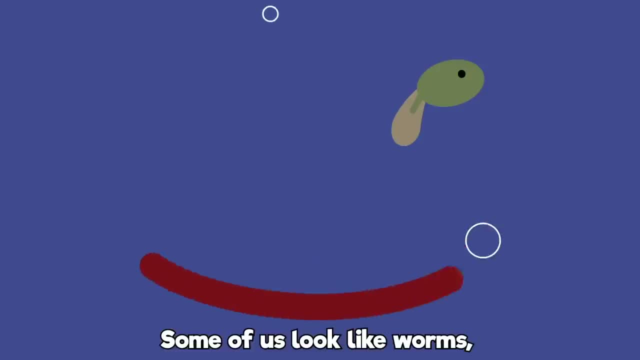 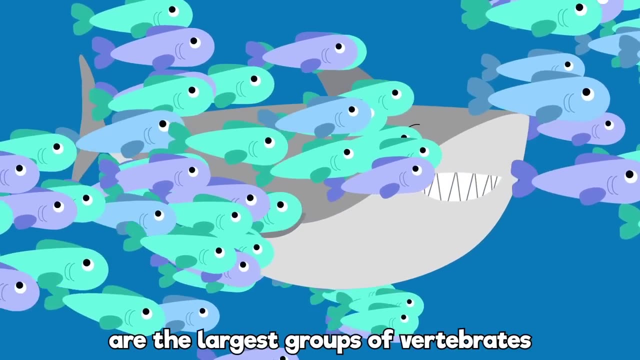 Some of us catch food with our specialized tongues. Some of us look like worms and some of us are long And some of us are toads, but most of us are frogs. Fish, fish, fish are the largest group of vertebrates.